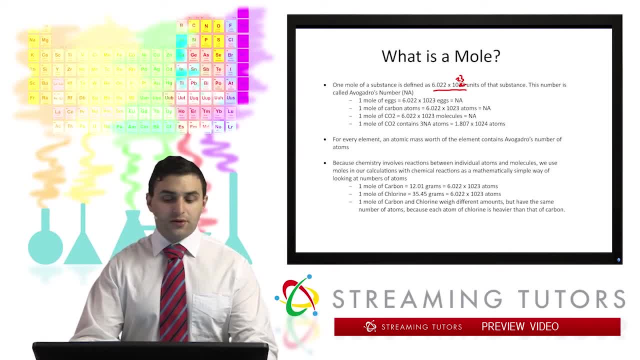 has a certain atomic mass. as we saw on the periodic table, An atomic mass worth of an element is known as atoms. A mole of that element contains Avogadro's number of atoms, As we see down below here. as I said before, chemistry involves reactions of atom versus atom and molecule versus molecule. 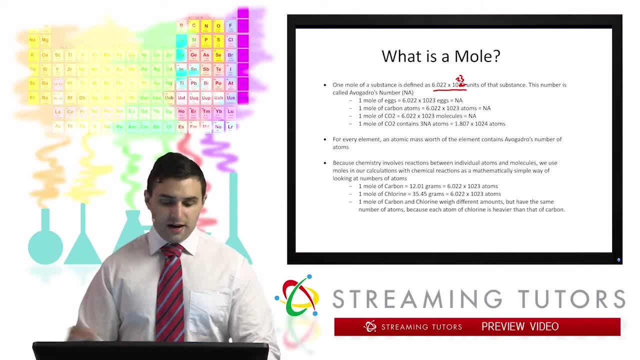 So what we see then is that one mole of carbon is going to weigh a different amount over here than a mole of chlorine, but they're going to contain the same number of atoms, And that's going to be useful when we're looking at stoichiometry and reactions, when we're 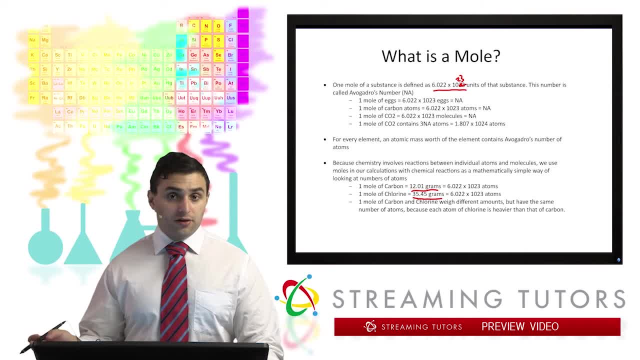 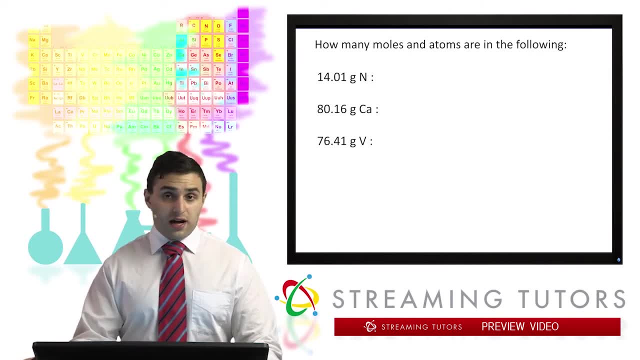 looking at how much of something reacts with how much of a molecule. So let's get into converting between grams and moles then, So we can look on the periodic table to get the atomic mass of each of these elements And we can convert it into moles based on how much of a certain element we're given. 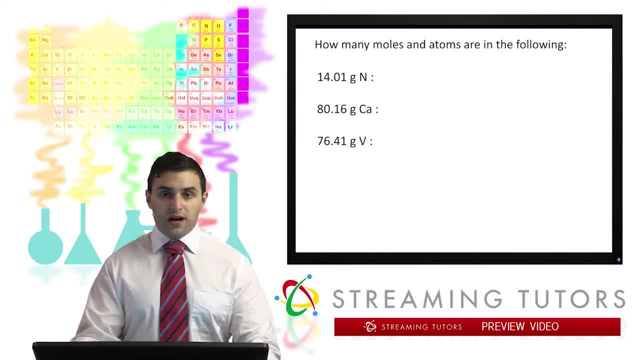 So, for example, first we have 14.01 grams of nitrogen. So if we look on the periodic table, we see that nitrogen has an atomic mass of of also 14.01 grams per mole. So what we're going to do, then, is convert in the following way: 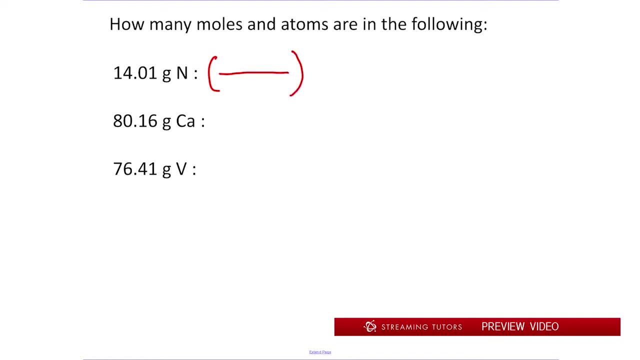 We're going to set up this little fraction over here On top. we're going to say that 1 mole of nitrogen contains 14.01 grams of nitrogen. What you see here, what we've done is we've just set up this little fraction which we 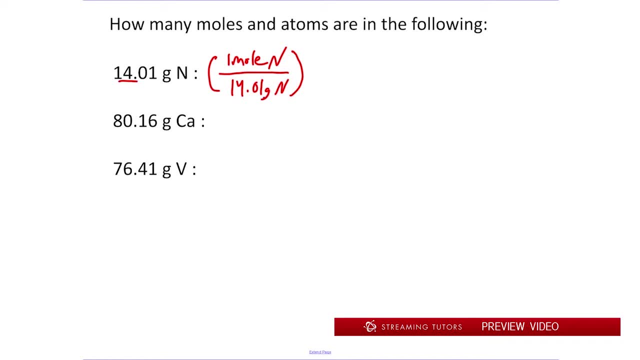 can multiply the original number by, We see that the grams of nitrogen cancel out and our final unit is simply going to be in moles of nitrogen. So if we do this, it's just equivalent to dividing by 14.01.. So that means we have one mole of nitrogen in 14.01 grams. Next thing: 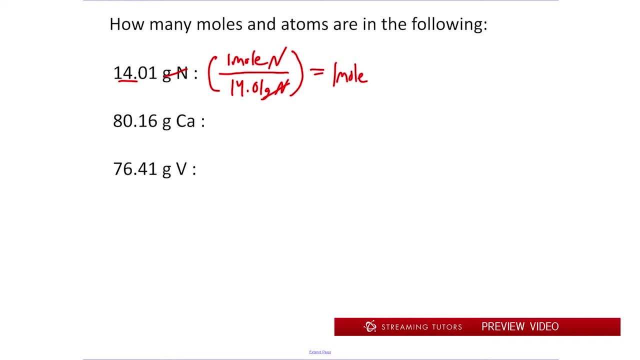 we can do is convert that then into how many atoms there are. So we're going to say that there's 6.022 times 10 to the 23rd atoms in every one mole of nitrogen, And so that gives us simply 6.022 times 10 to the 23rd atoms of nitrogen. So that's a nice easy. 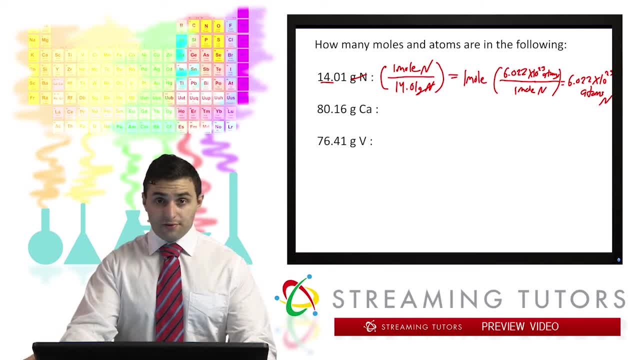 foolproof way to convert When we use this fraction over here, as we did over here. that's going to make sure that our units are canceling out correctly, making sure that we're not multiplying when we should be dividing or dividing when we should be multiplying, And 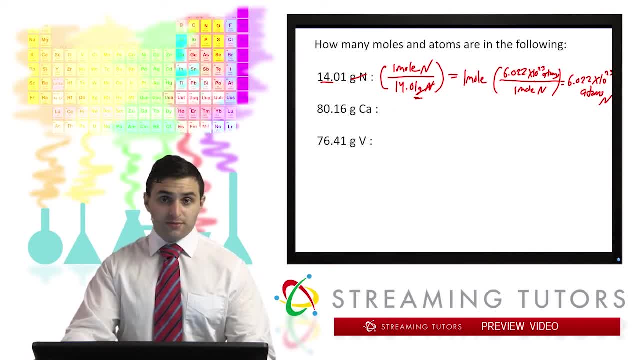 you can use this for any kind of conversion from grams to moles, moles to grams- what have you? So let's take a second to pause the video, see if you can do the next two on your own, Okay. 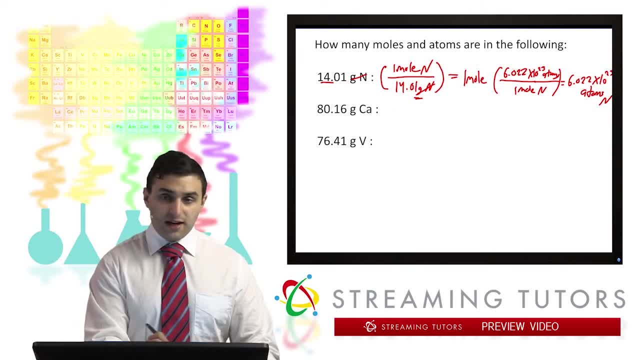 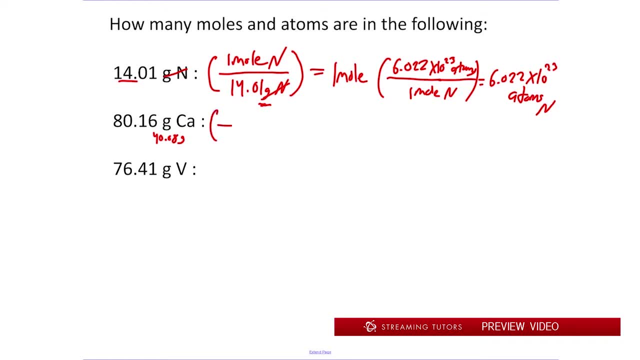 so let's look at the second one, for calcium. So, for calcium, calcium has an atomic mass of 40.08 grams. So what we're going to do, then, is we're going to do the same thing we did for nitrogen: We're going to say that one mole of calcium contains 40.08 grams of. 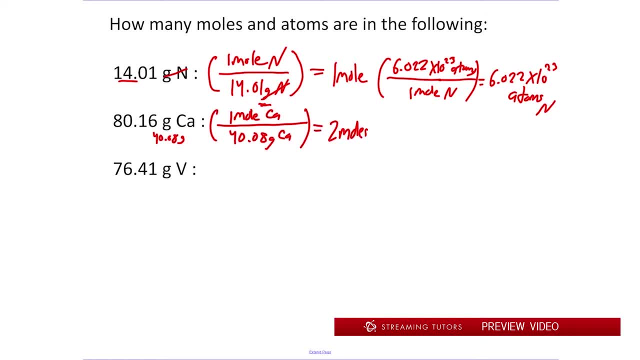 calcium. So that means we have two moles of calcium. Then we're going to convert that into how many atoms there are the same way, And so that gives us two times Avogadro's number of atoms in this sample of calcium. That number 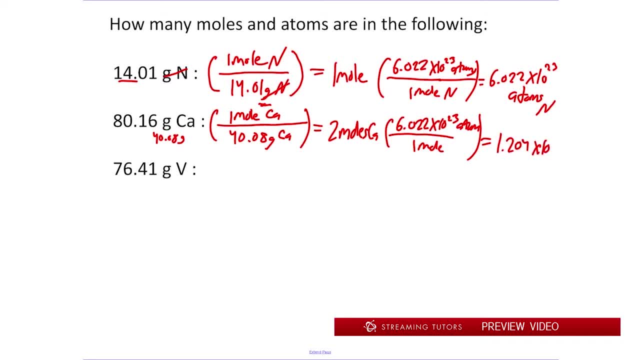 turns out to be 1.204 times 10 to the 24th atoms of calcium. And then finally, for vanadium. vanadium has an atomic mass of 40.08 grams, So that means that we have two moles of calcium. 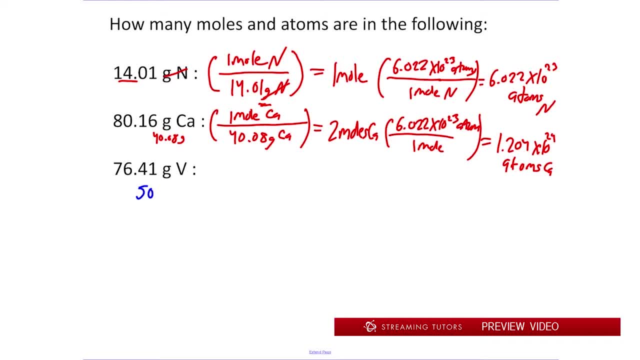 in this sample. So what we're going to do then is we're going to say that one mole of vanadium contains 50.942 grams. So we do that and we get 1.494 moles of vanadium. Next we're. 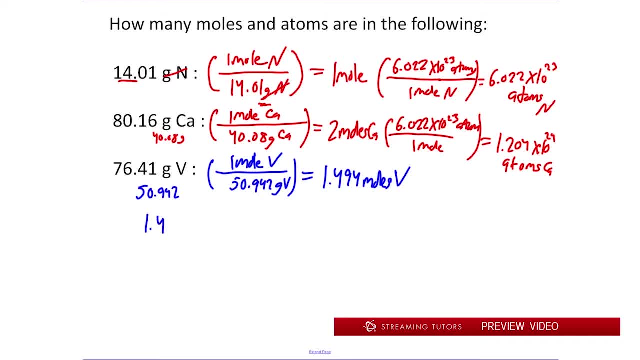 going to convert that into atoms, the same way we've been doing before. multiply by Avogadro's number, So this many atoms in one mole of compound. We see that moles cancel out here and we're left with 9.0 times 10 to the 23rd atoms of vanadium in that sample. So doing this is 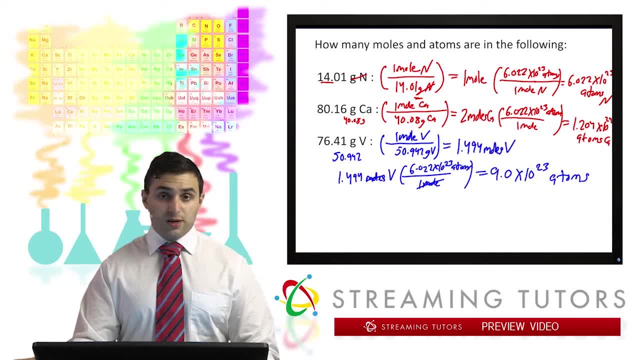 going to be extremely important in the future: Converting from grams to moles, back from moles to grams, which we'll do in one of the next slides. So it definitely takes its time to practice doing this and make sure that you're able to do it without making or arithmetic. 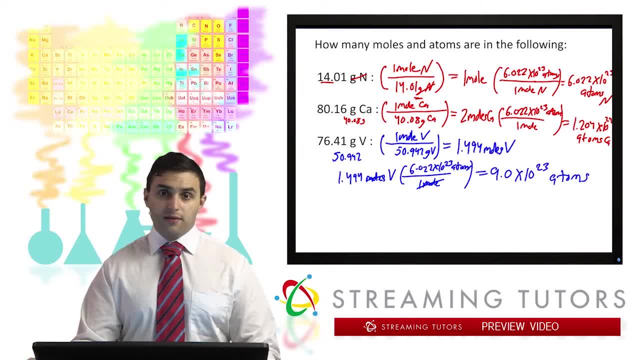 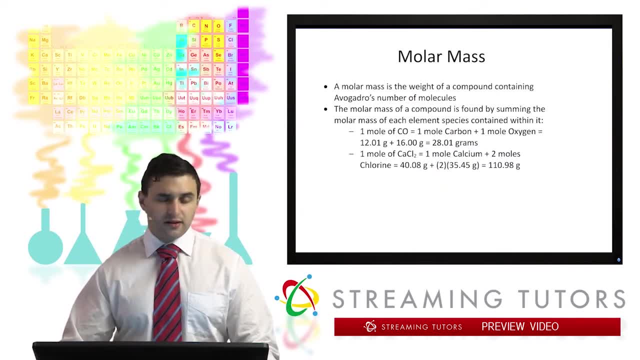 errors. Okay, so let's move on to the next slide, where we're going to talk about something called molar mass. So a molar mass is going to apply to both atoms and compounds. A molar mass is just the weight of molecule or weight of a compound that contains Avogadro's number. 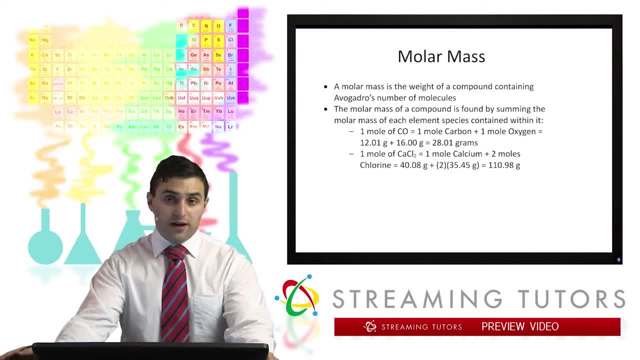 or the weight of one mole of compound. So the molar mass of a compound can be determined based on the molar masses of the elements it's comprised of. For example, down here we have carbon monoxide, over here We said it contains. 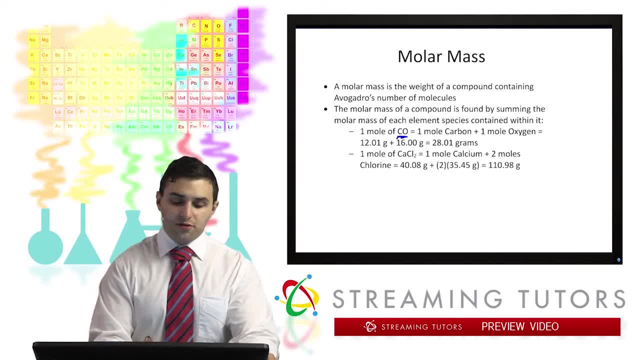 if we have one mole of carbon dioxide, that means we also have one mole of carbon and one mole of oxygen. So to find the molar weight of carbon monoxide, CO, all we have to do is just add up the molar weight of carbon. 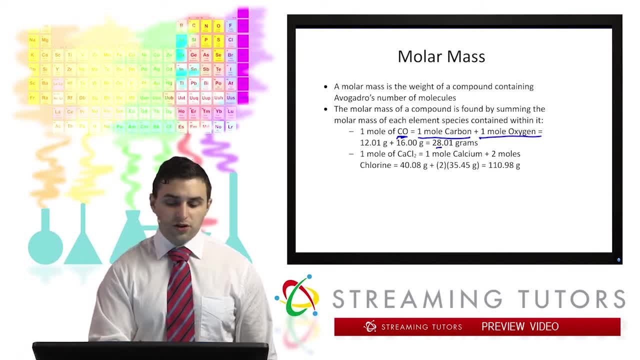 plus the molar weight of oxygen, and that gives us a total of 28.01 grams. We can do the same thing for a compound like CaCl2.. One mole of CaCl2 has one mole of calcium as well as two moles of chlorine. 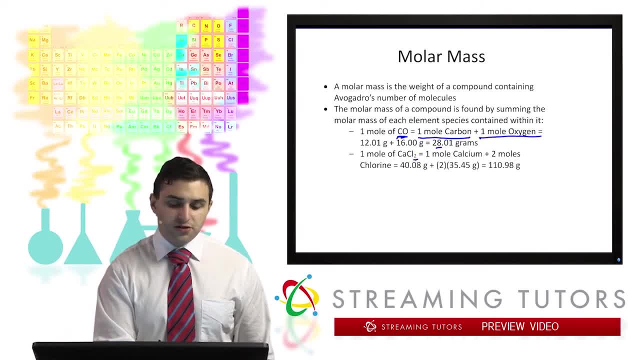 You'll note that it has two moles of chlorine because of this 2 at the end of the stoichiometry of the molecule. So we're gonna do the same thing there, just add up the molar weight of a carbon monoxide. One mole of CaCl2 plus two times the molar weight of chlorine, So that gives us a final molar weight of 110.98 grams. Finding the molar mass of a compound is pretty straightforward, but it's also gonna be an extremely important thing. 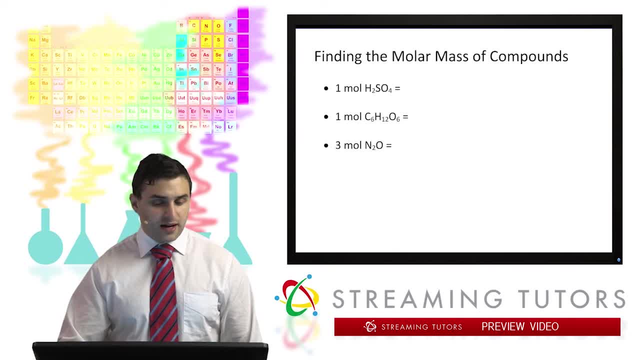 to be able to do So. let's take the time and try and find the molar mass of some compounds. Once again, pause the video and try these out on your own. See if you can add up all the atoms to find the molar mass. 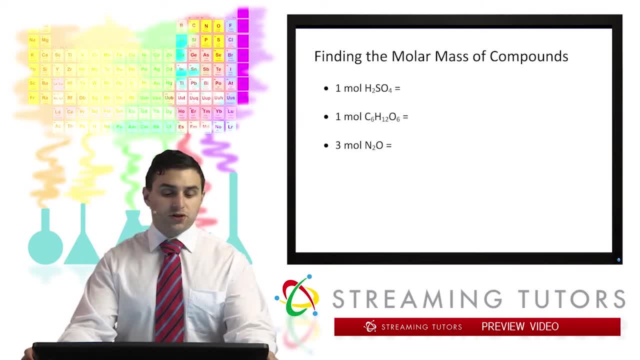 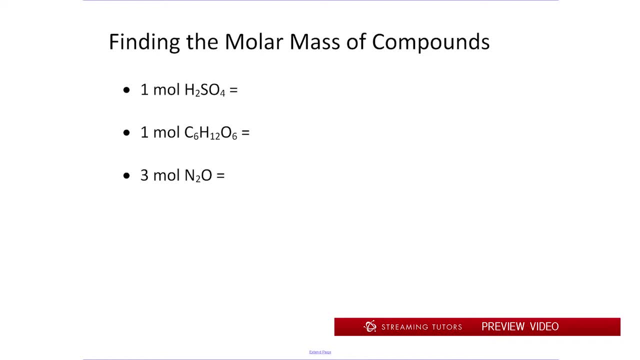 Okay, so let's look at the first one. First we have H2SO4.. So that has two moles of hydrogen, one mole of sulfur and four moles of oxygen. So we're gonna have something like this: We have two hydrogens times a molar mass of about one.